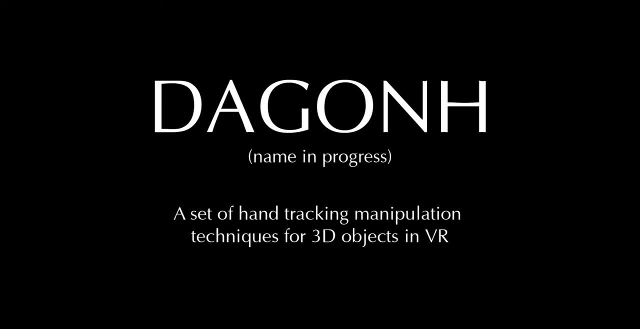 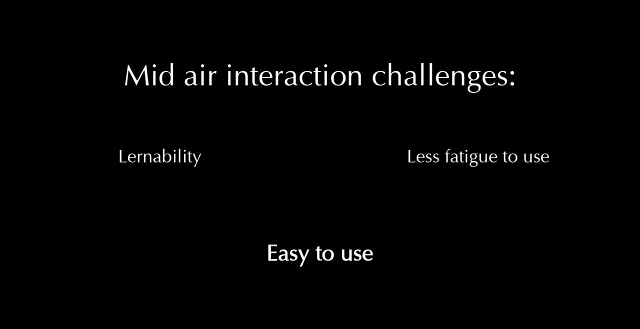 TEIKUN is a set of interaction techniques for the manipulation of 3D objects in a virtual environment, using hand tracking technology as input. The proposed techniques aim to address the constant challenge of mid-air interactions: learnability and less fatigue to use. Hand tracking and gesture recognition provide a metaphor that has the intention to be easy. 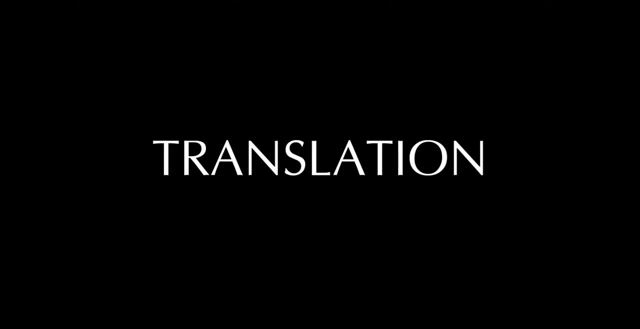 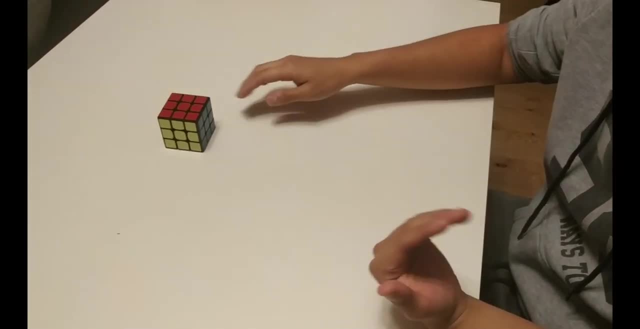 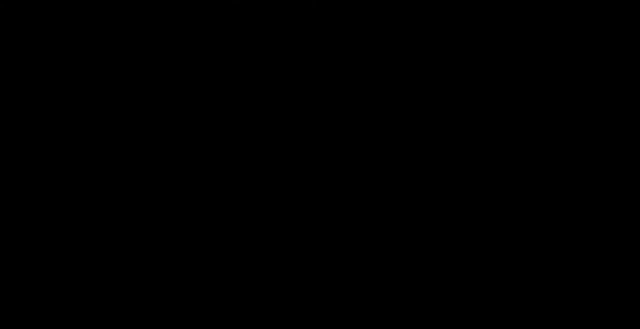 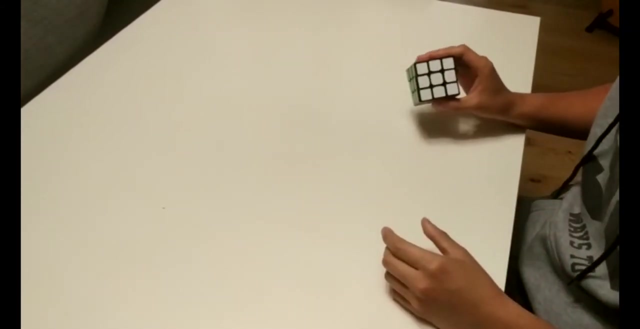 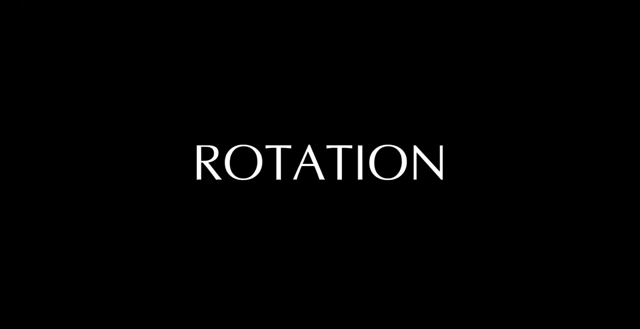 to perform by users. Objects selected at a distance can be approached to the user using intuitive gestures that will be performed with the opposite hand of the selection. Alternatively, remotely selected objects can be positioned at the location of the hand that made the selection, and translation can be performed between both hands. 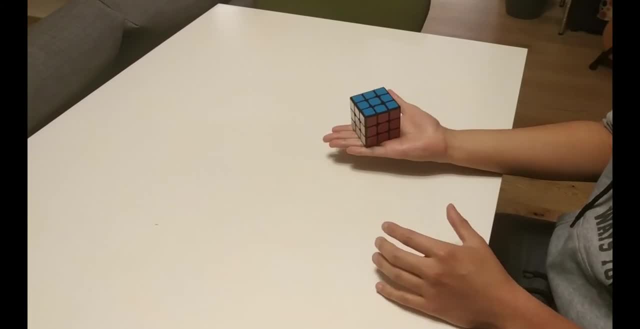 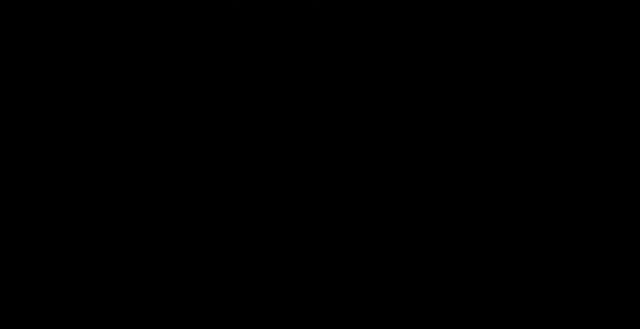 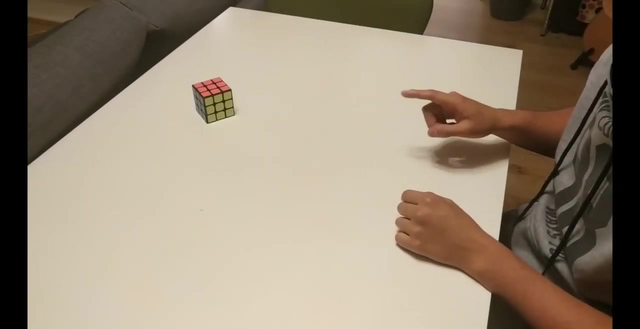 Users can activate rotation holding an object and move their hand facing up. Releasing the object will deactivate its gravity, making it easier to manipulate with the other free hand. Objects selected at a distance can change their size. Objects selected at a distance can change their size. 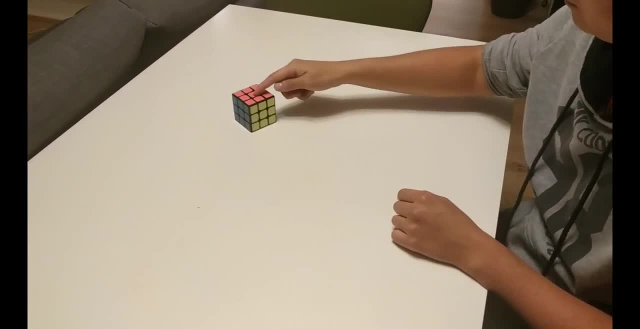 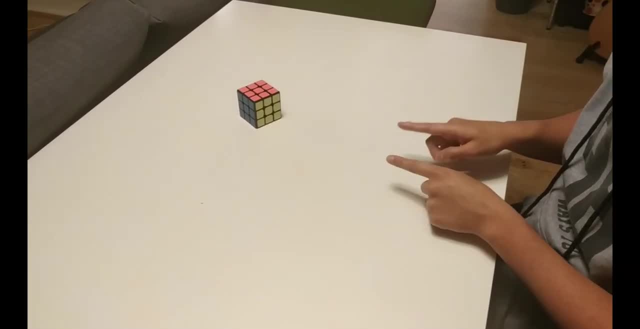 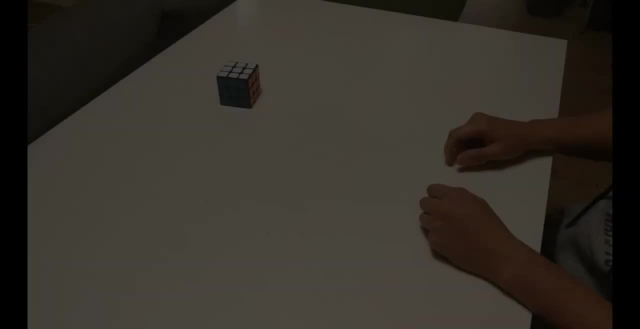 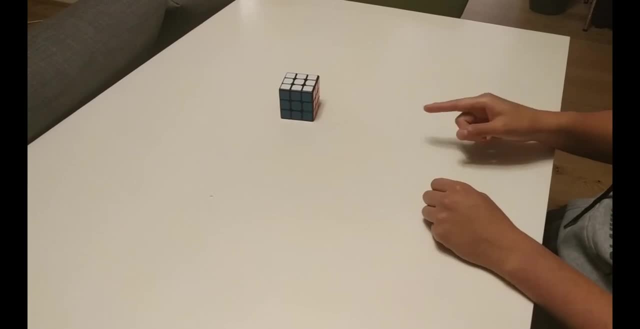 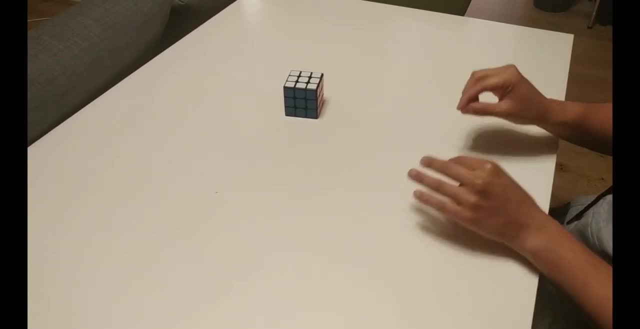